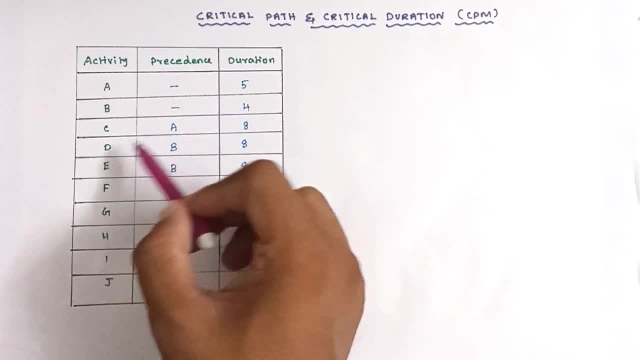 a, so for c, for a, the precedent activity. so the precedent relationship that is called the c activity is started when the a activity is completed. so after the completion of b activity, d activity will be start. so likewise in every activity having the precedent relationship. so first we have to draw the network path. so first we have to draw the network path. so 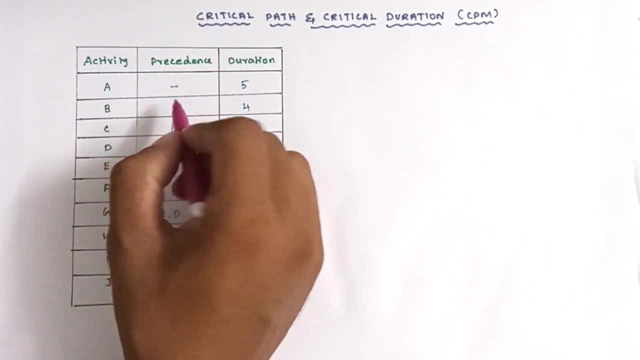 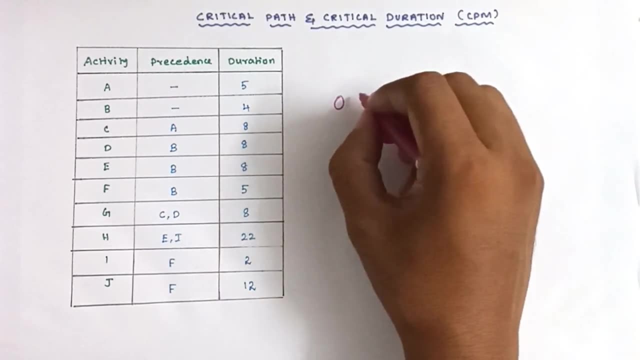 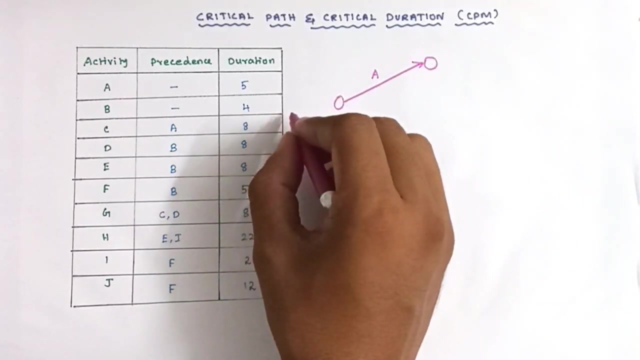 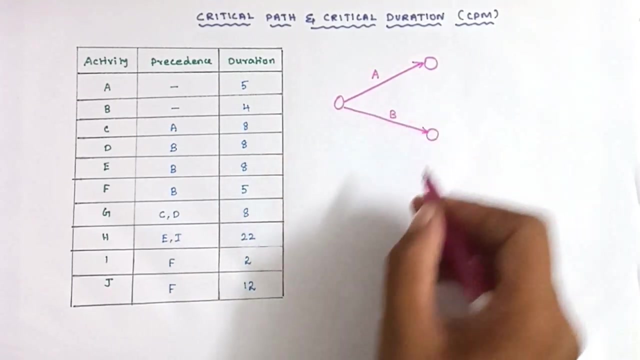 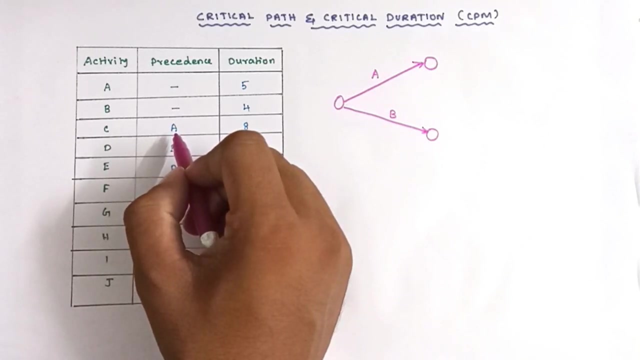 so first the for A and B. there is no precedent relationship, so we can draw A and B. ok, so the A activity. so there is no precedent activity. so next one is so B, so B also having no precedent activity. so next we have to draw C activity. so after completion of A activity, C will be. 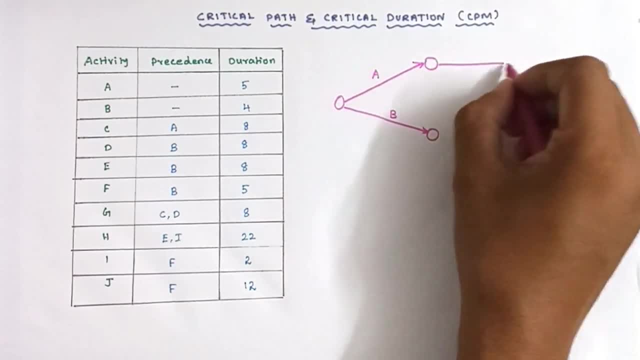 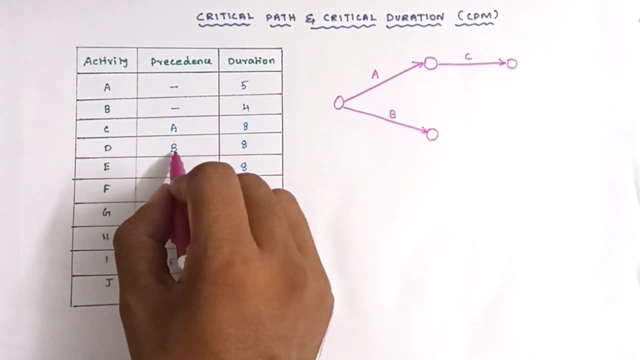 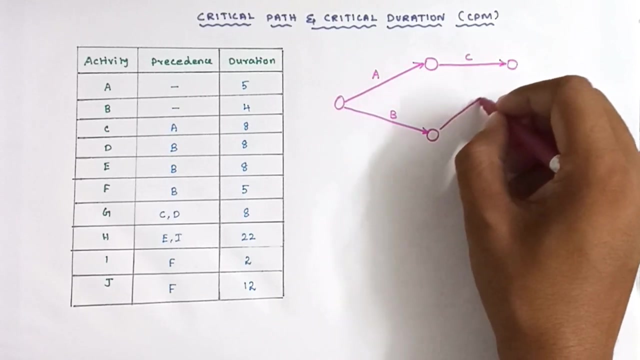 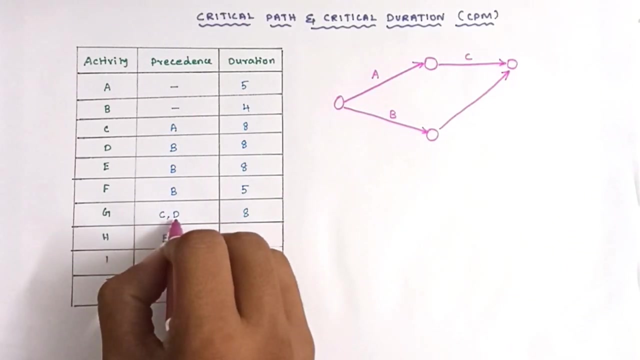 start. so after A, C activity will be start B activity, so B activity will be start after the completion of B activity. so we can draw B activity. so we can draw over here because of in 0, G, C and D is the present relationship, So so we can put D. So after completion of C. 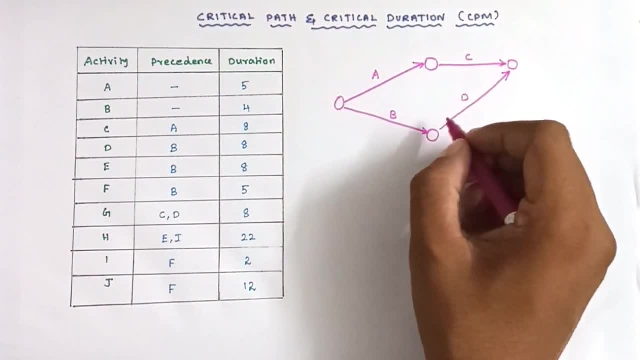 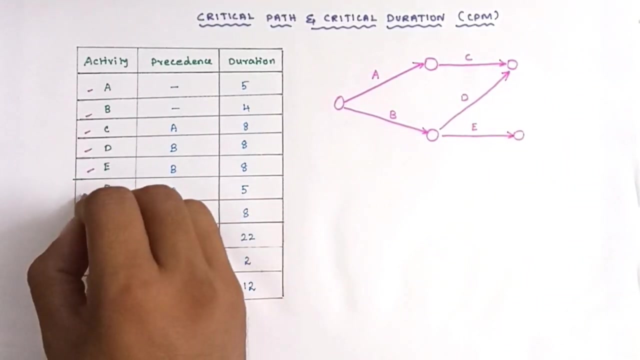 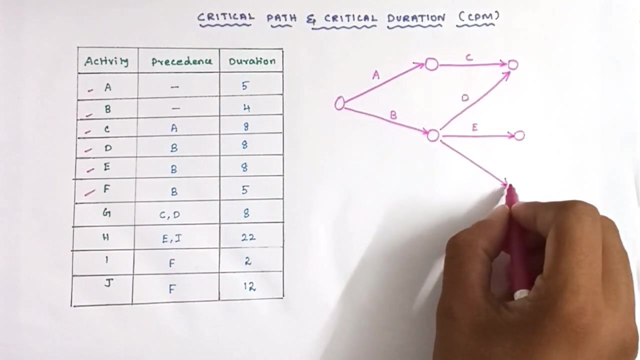 and D, G will be started. So again, so we can draw this. So next E activity. So we can draw the E activity. So E. So next F. So F, also having the present relationship of B, So we can draw over. here is F activity. So next we have to draw the G activity. So 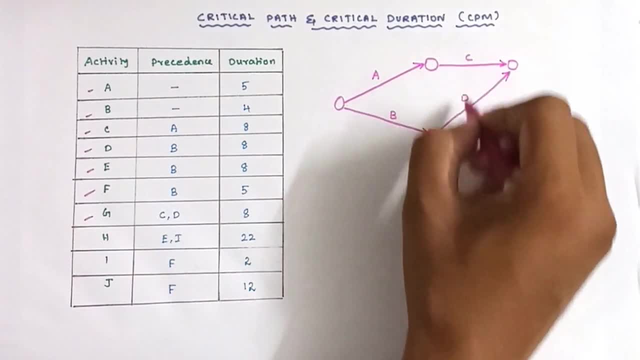 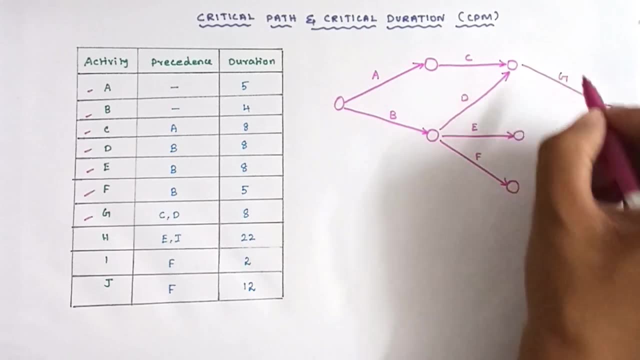 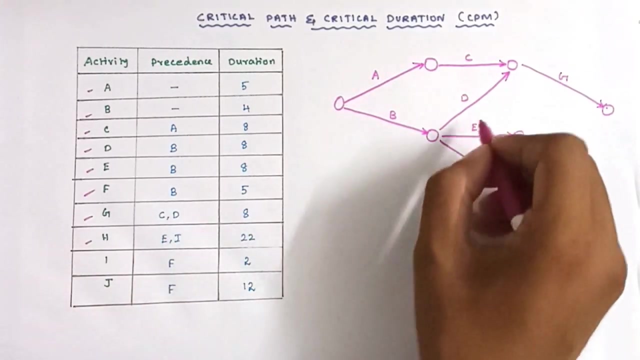 C and D is the precedence, So C and D, So we can draw G activity, So after that H activity. So we can. we need to the present relationship E and I. So there is no I over here. So 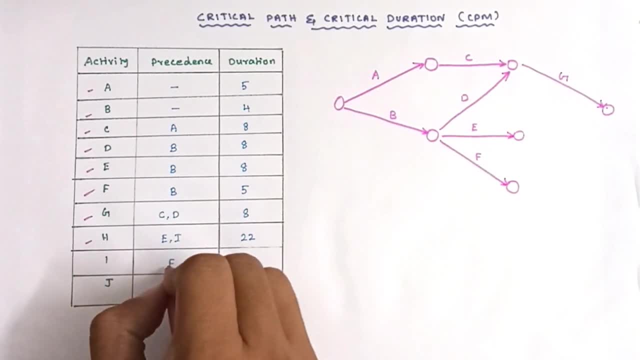 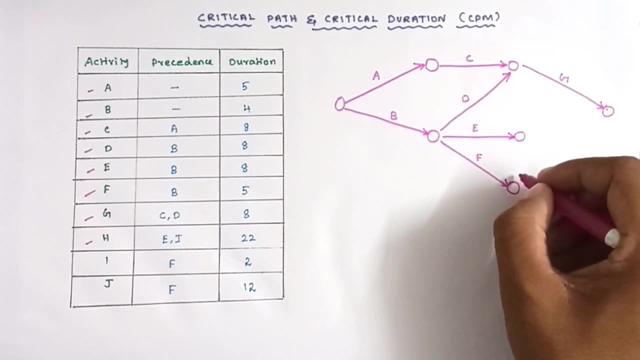 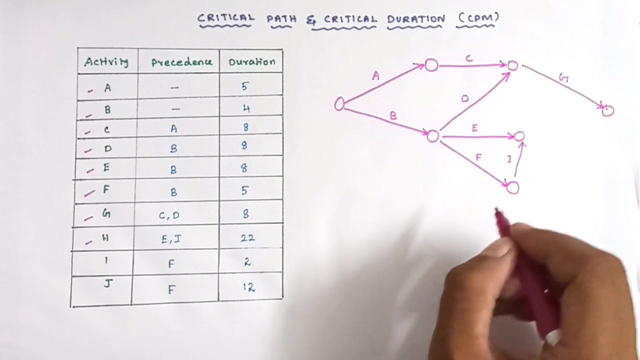 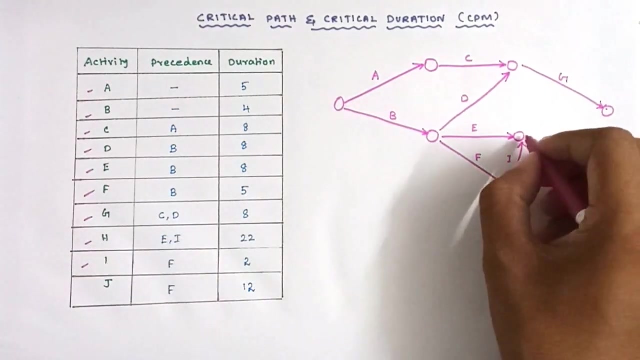 we can. first we have to draw the I activity. So the I precedence activity is F, So we can draw I value. So E and I is the precedence activity of H. So we can draw over here. So I activity, So for H activity, So E and I is the precedence relationship. So 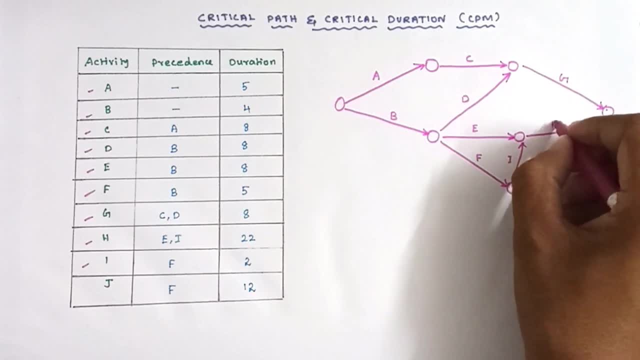 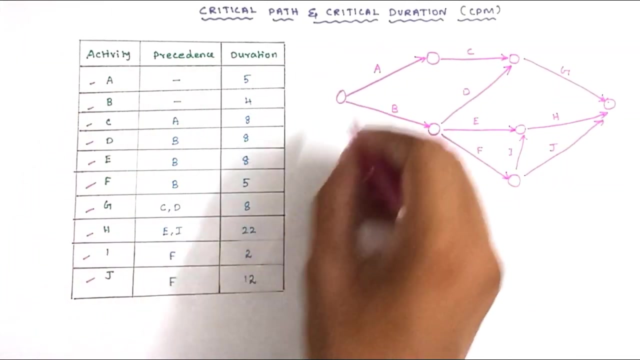 we can draw H over here, So H activity. So then for J activity the precedence is only F, So we can draw over here. So in corresponding activity we can put the duration value, So A equal to 5 and C is for 8, and. 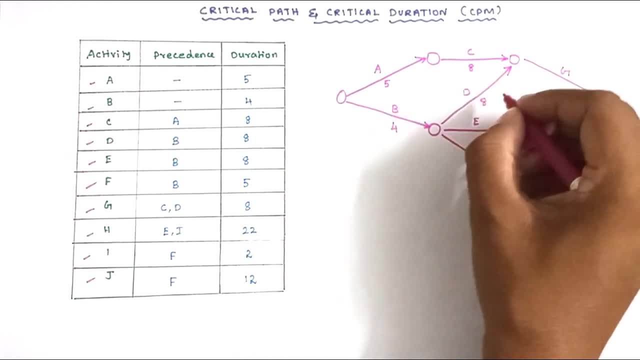 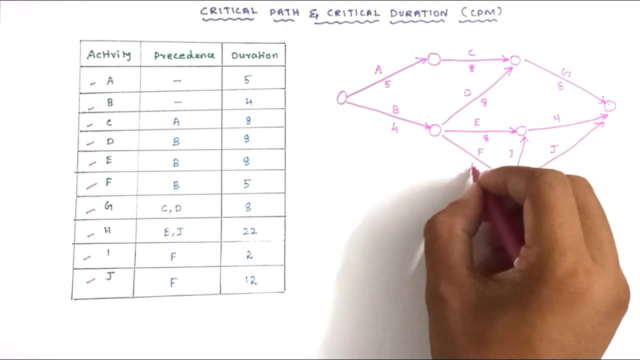 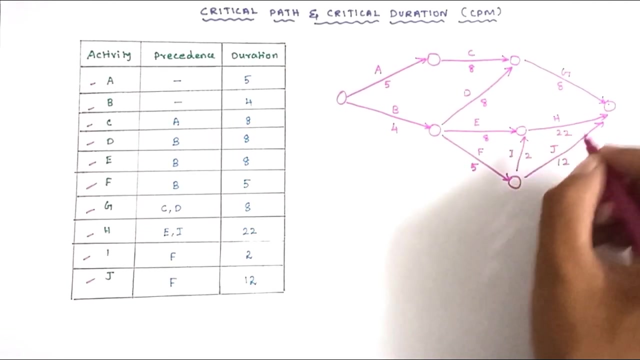 B is for 4.. Then D is equal to 8 and G is equal to 8. So for E, duration is 8 and F value is equal to 5. Then D is equal to 2 and J is equal to 12 and for H is equal to 22.. So this is how we can. 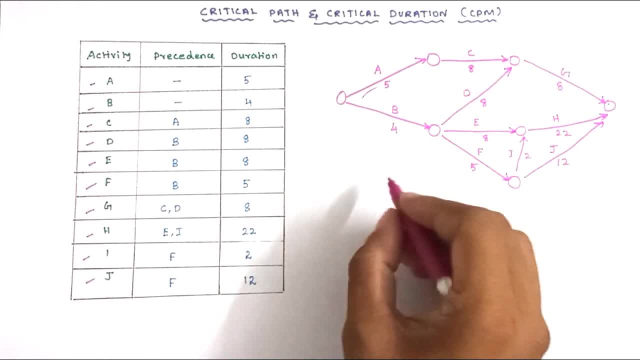 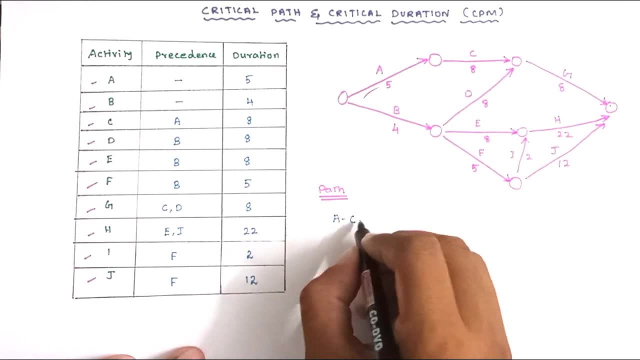 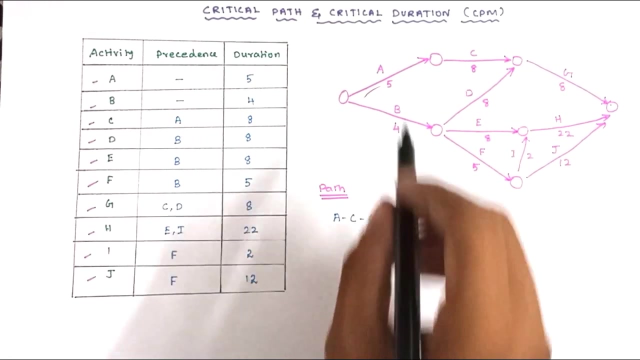 draw the network path. So after that we have to calculate the path. So path: So A, C, G is one path. So A, C and G. So A and C, G is one path. So next, B, D, G. So B, D. 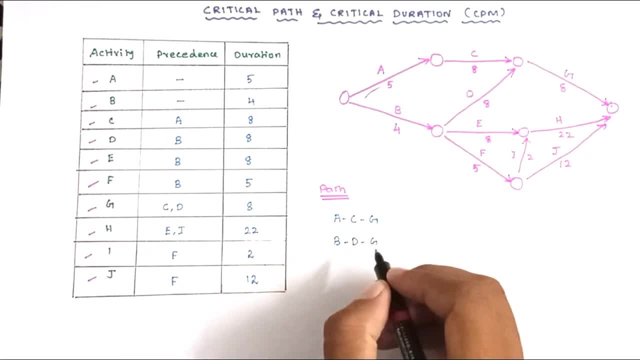 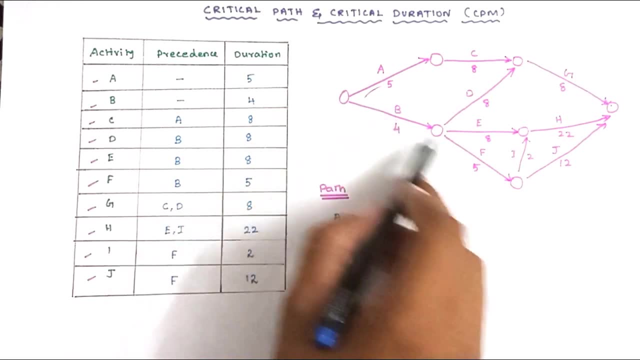 G, G, Okay, so next B E, H. So next B F, J. Okay, So next B F, I H. And the all of a sudden, Wenn I can, you can. to find out one path, double click. 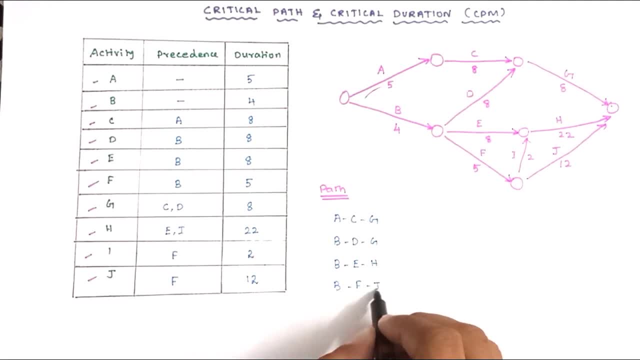 So next B, F, J. If that's B, G, G, How do I do that? OK, So let me just take one path. So B E, H. Next I did B, F I H. So that's, that's just an index two. 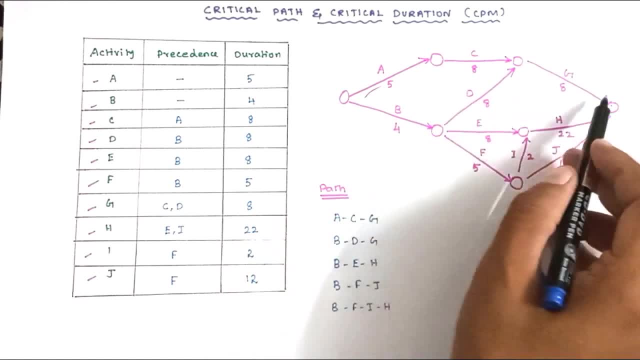 Next B, So B, E, H, So T. So next B N D G and B D G. So now next B, F, I, H. So that's IB F I. the method is it's used for: 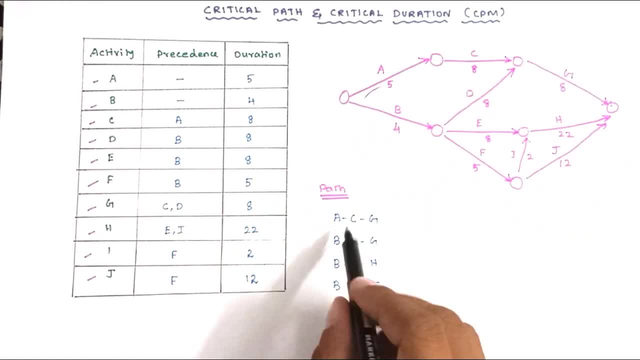 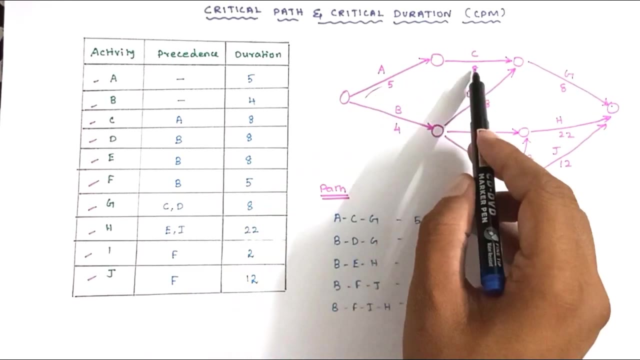 and BEH. so everything is calculated. so 1, 2, 3, 4, 5, so there are 5 paths in this network diagram so we can put the corresponding durations 5 plus 8 plus 8. so because the 5 plus 8 plus, 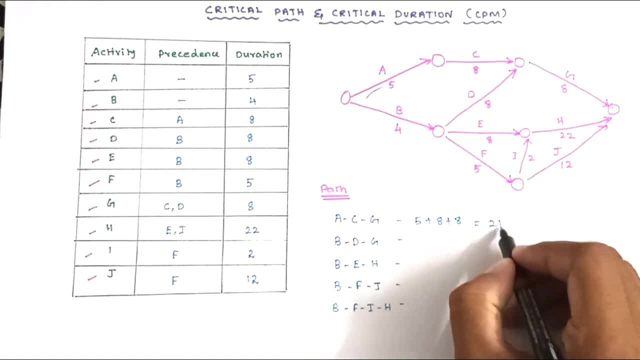 8, so the total value is 21, and BDG, so 4 plus 8 plus 8, so the value is 20, and then for BEH, so 4 plus 8 plus 22, so the value is 34, and BFJ, so BFJ is equal to 4 plus 5 plus 12, equal. 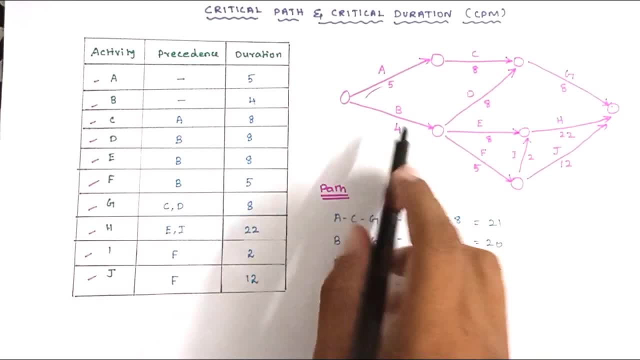 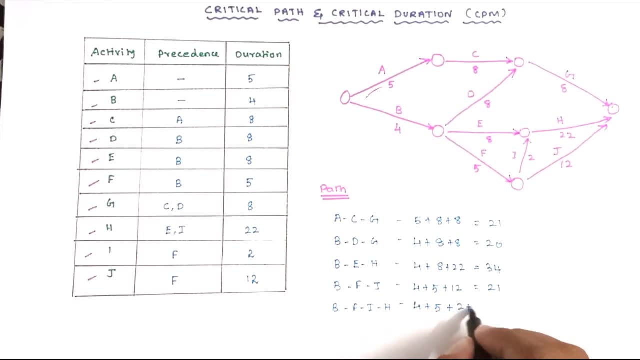 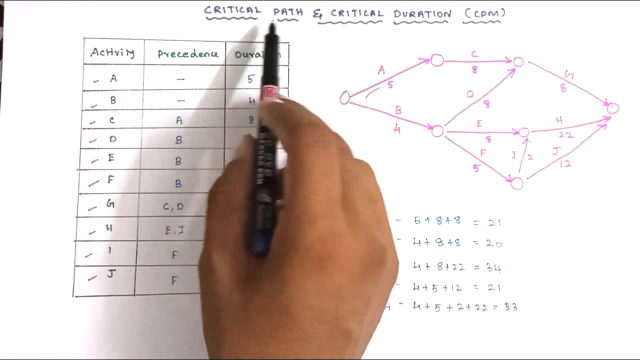 to 21. so then BFIH, So BFIH. so 4 plus 5 plus i is equal to 2 plus 22, so the value is 33. so we already said the critical path and the critical duration, though the path having the longest duration, that 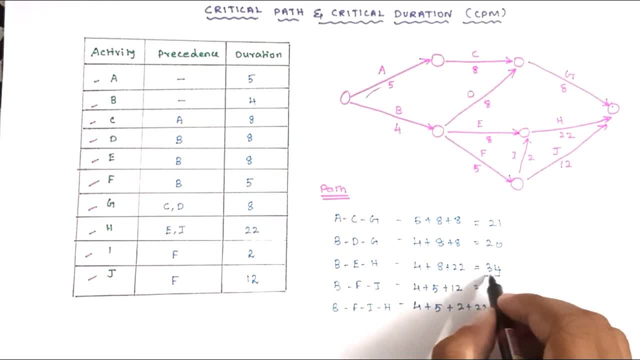 is called critical path. so the longest duration path is 34, so this is the longest duration and path is equal to BEH. So this is the critical path and this is the critical duration. so this is a method to solving the problem. The problem related with the critical path and critical duration. so that is critical. 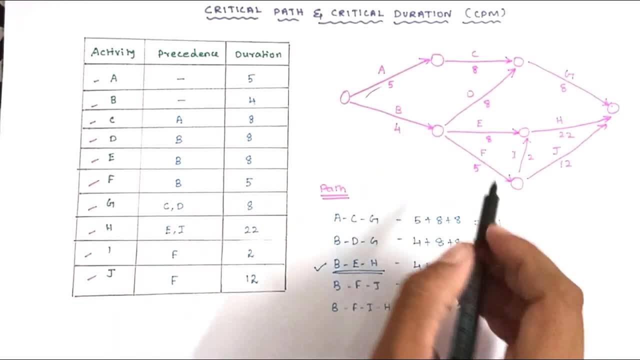 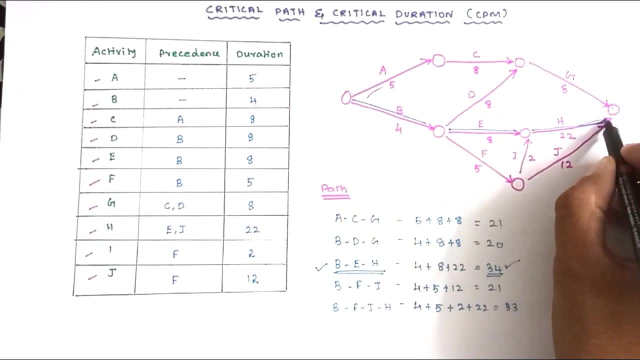 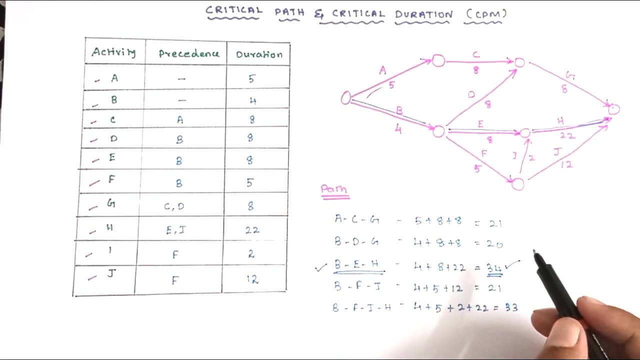 path method. so we can highlight the critical path, so BEH. so we can highlight BEH. so this is the critical path and the critical duration is 34. so again, we will see in next problem. thank you. 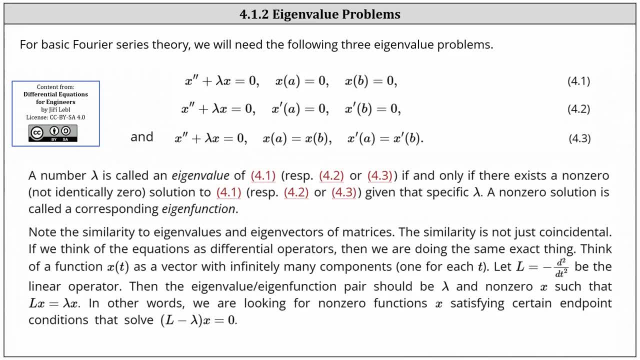 In this lesson we'll find the eigenvalues and eigenfunctions of a given boundary value problem. For basic Fourier series theory we'll need the following three eigenvalue problems: For 4.1, we have x, double prime plus lambda. x equals zero where x of a and x of b equals zero. 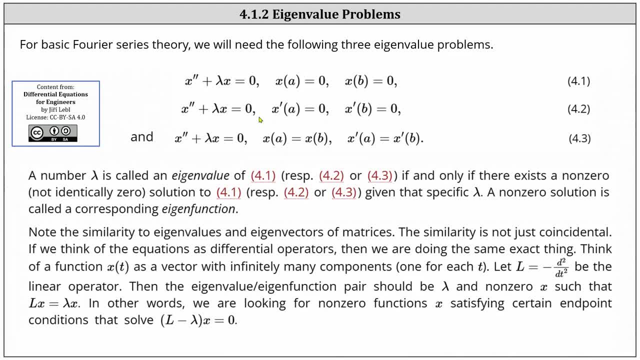 For 4.2, we have x double prime plus lambda x equals zero, where x prime of a and x prime of b equals zero. And for 4.3, we have x double prime plus lambda x equals zero, where x of a equals x. 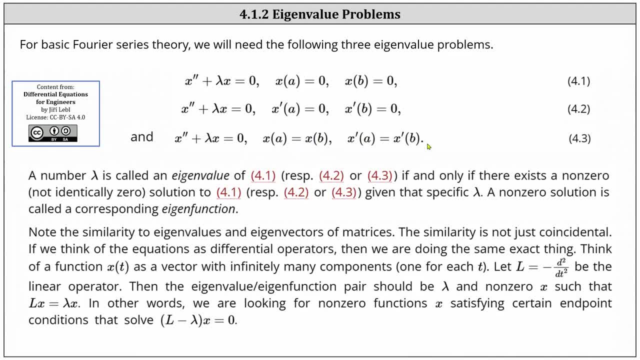 of b and x. prime of a equals x prime of b. A number lambda is called an eigenvalue of the boundary value. problems 4.1 through 4.3, if, and only if, there exists a non-zero solution to the problem. given that specific lambda, A non-zero solution is called a corresponding eigenfunction.